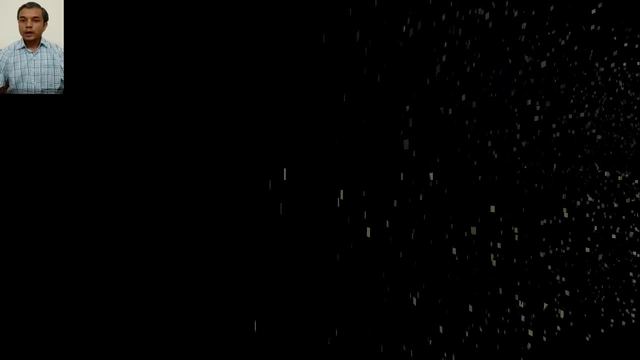 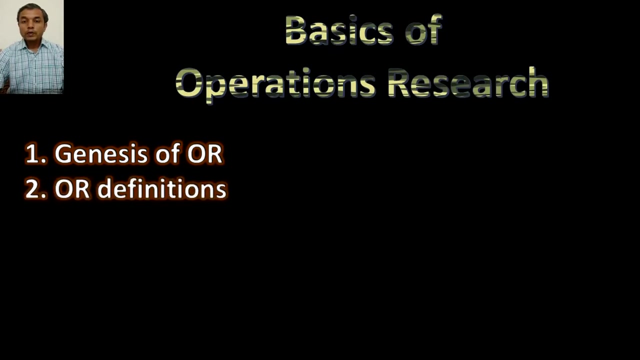 Hello students, Today we will discuss basics of operations research. During this session, we will discuss genesis of operations research, how operations research is evolved, various definitions of operations research, characteristics of operations research, various phases of operations research, models and models used in operations research. 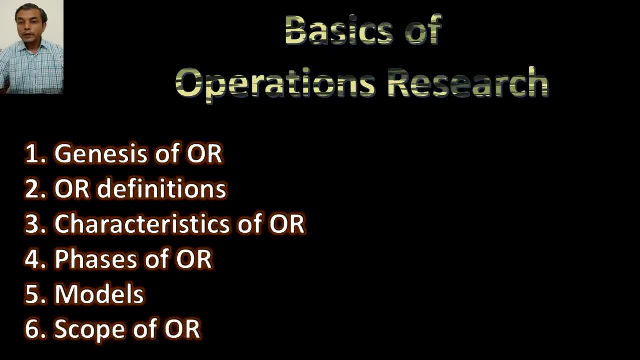 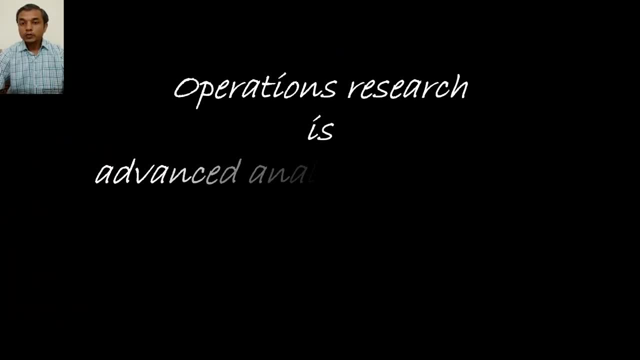 and scope of operations research and applications of operations research. Let's start with basic definitions of operations research. What is operations research? Operations research is advanced analytical methods to help make better decisions, So operations research is a useful tool to managers to take better decisions. 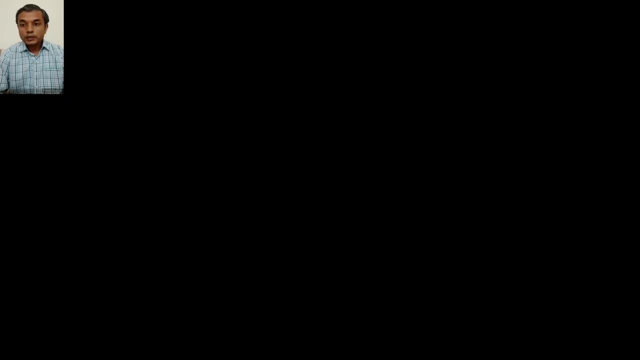 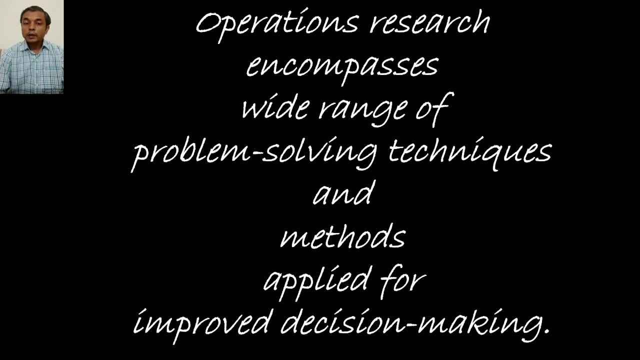 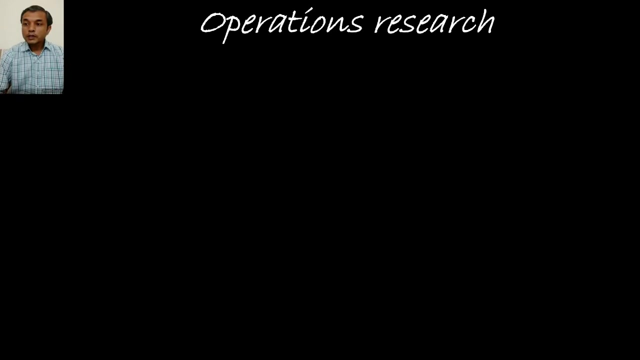 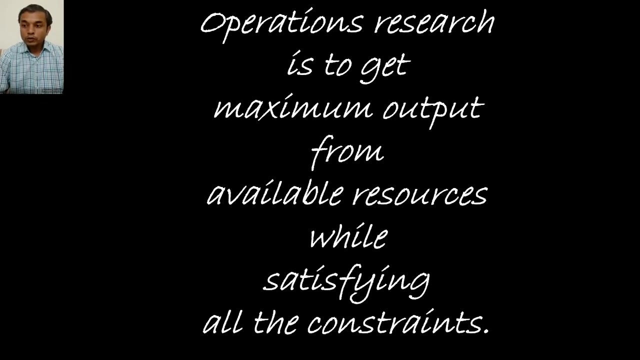 It is also said that operations research encompasses a wide range of problem-solving techniques and methods applied for improved decision-making, So operations research is nothing but a bunch of optimization techniques that is used for making better decisions. It is also known as optimization techniques. Operations research is also known as to get maximum output from available resources while satisfying all the constraints. 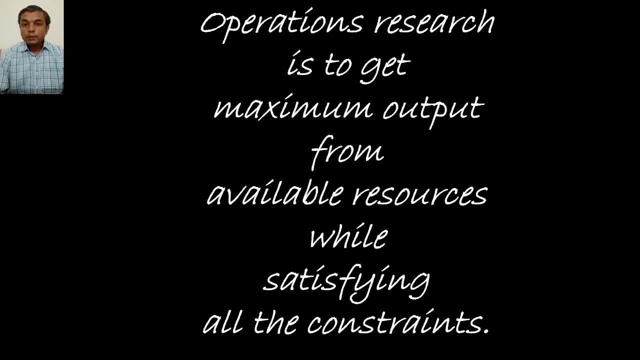 So, since the beginning of the humankind, we are always facing scarcity of resources and also surrounded by so many constraints. Same scenario is observed in industries, So operations research is a tool that provides maximum output from the given the resources while satisfying the all constraints. 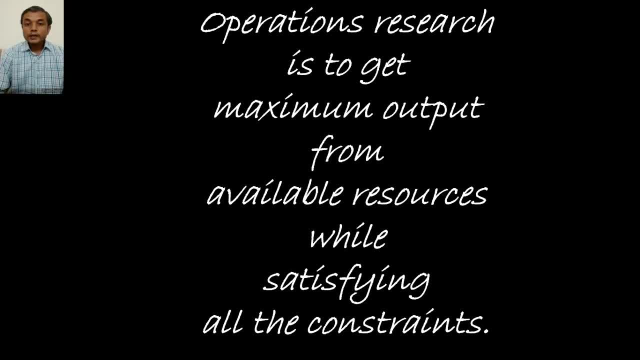 So, in short, we can say that operations research is a decision-making tool that is used, that is used by managers for getting maximum output from the available resources, satisfying all the constraints. operations research is a bunch of optimization techniques, so the first question arise is that it's a bunch of 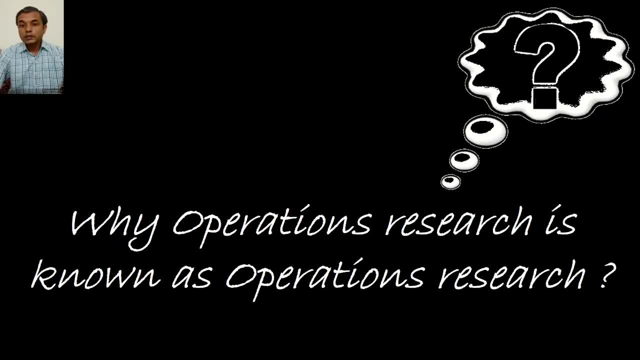 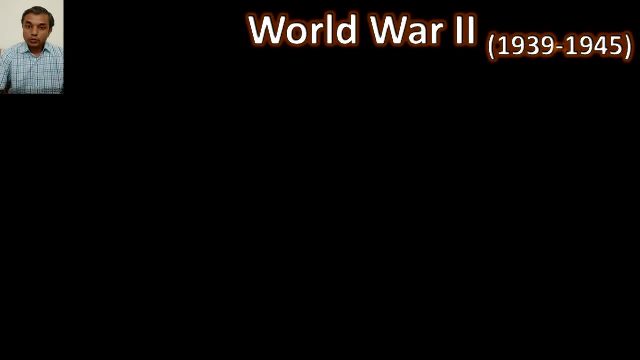 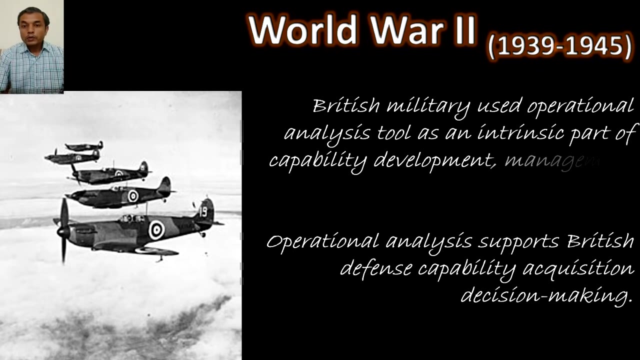 optimization techniques. let's see why operations research is known as operations research. actually, operations research is a war baby. during World War two first time British military used operational analysis tool. so in operational analysis tool they use for Air Force, Navy and army. so British military used to operational analysis tool as an intrinsic part of capability. 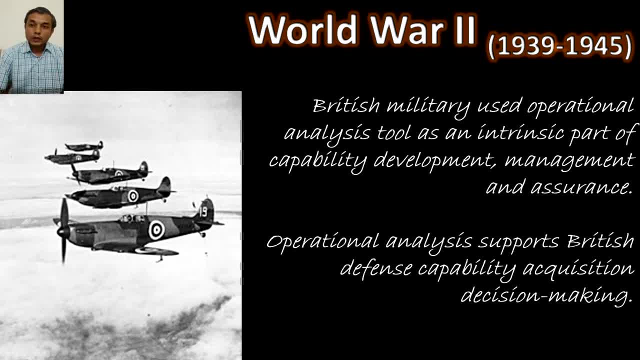 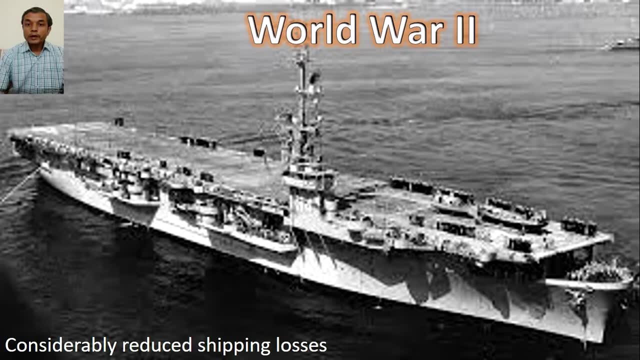 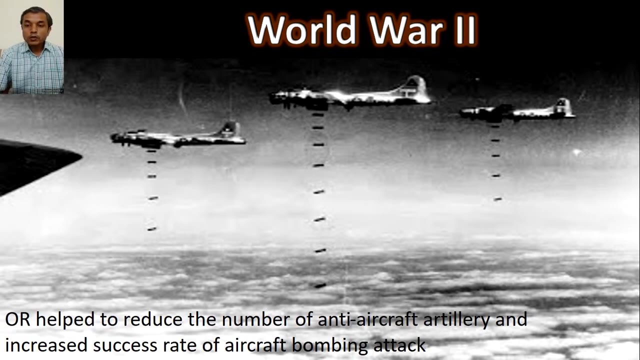 development, management and assurance. operational analysis supports British defense capability acquisition and decision-making. with the help of the operational analysis tool, British military has make so many decisions in more, better way in Air Force services operations. research has to reduce the number of anti aircraft artillery and increase the success rate of aircraft bombing attack by help of. 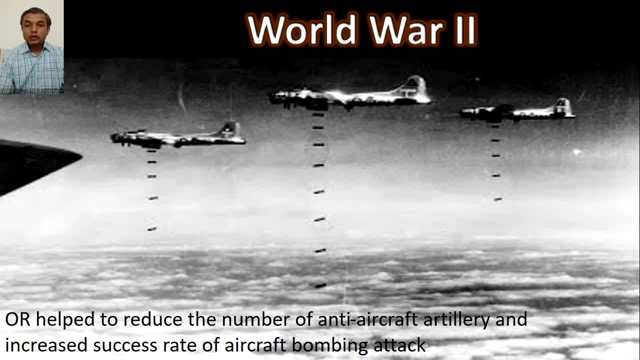 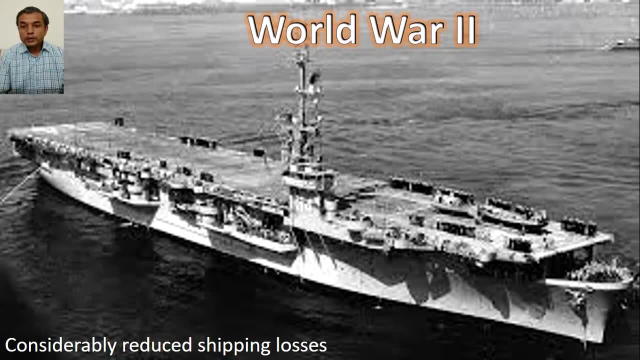 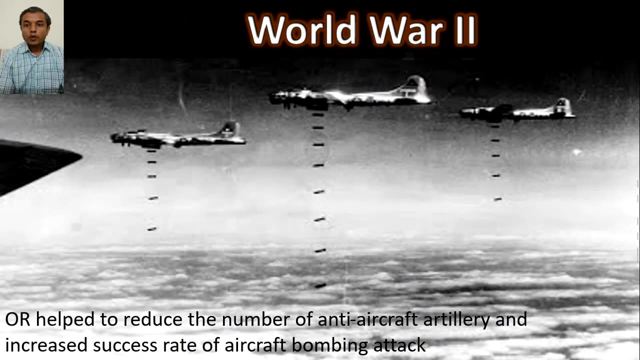 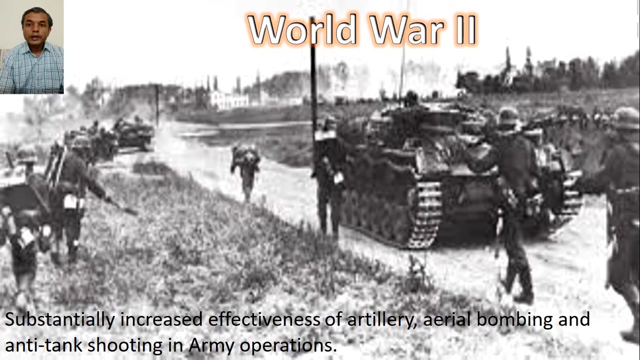 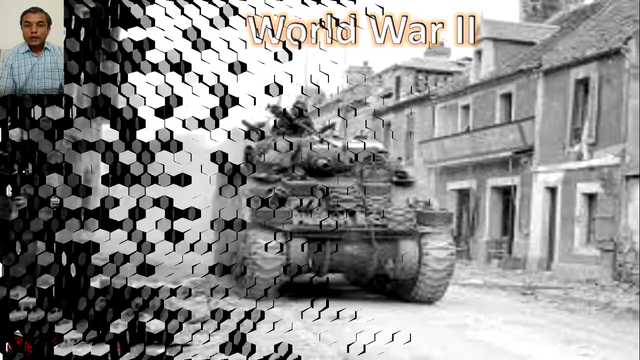 the numerical techniques. they increase the success rate of aircraft bombing attack. it is also used by Navy and by use of operations bay use. the purposes research techniques, the considerably reduced shipping losses in army operations, the substantial increased effectiveness of artillery aerial bombing and anti-tank shooting in army operations. so British military has 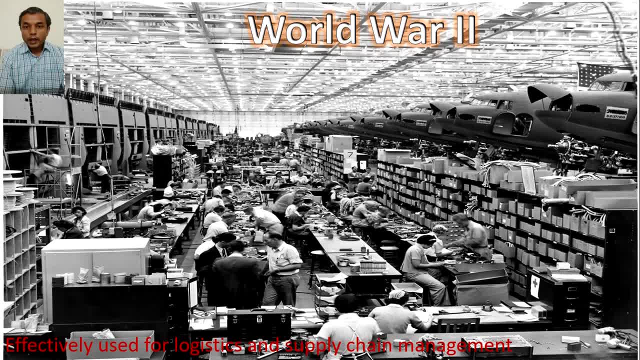 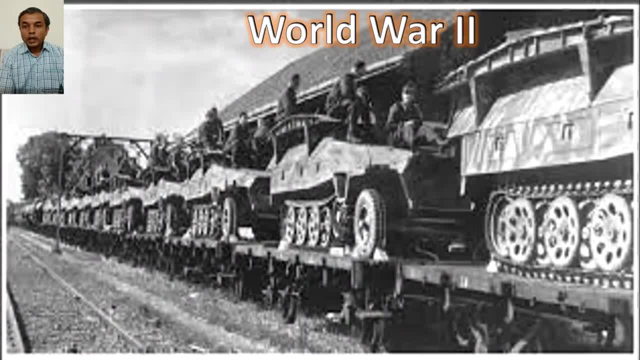 not only use operations research techniques for air force, navy and army, but they also used for supply chain management and logistics and by use of these techniques british army, with british military, performed very good in world war ii by very less resources and so many constraints. so this is why the name is operations research, as the majority of optimization techniques are. 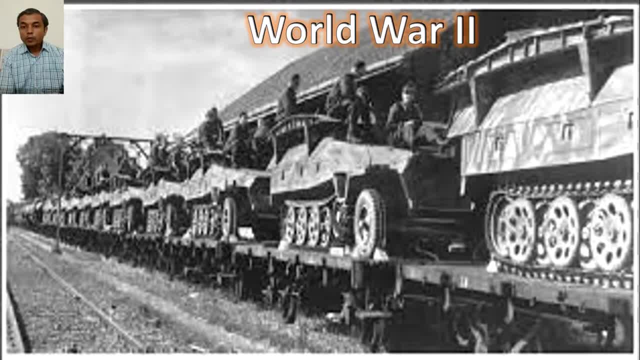 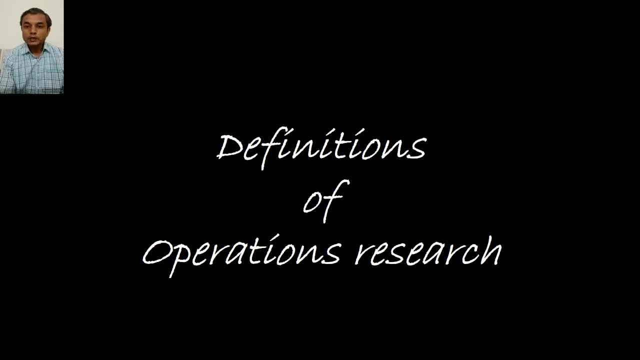 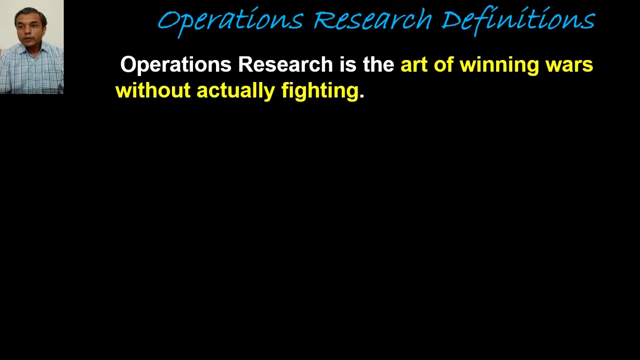 developed during the world war ii. in fact, so many techniques of operations research are also used before a world war ii, like inventory control. so now next is definitions of, or let's see few definitions of, operations research. first is operations research is the art of winning wars without actually fighting. 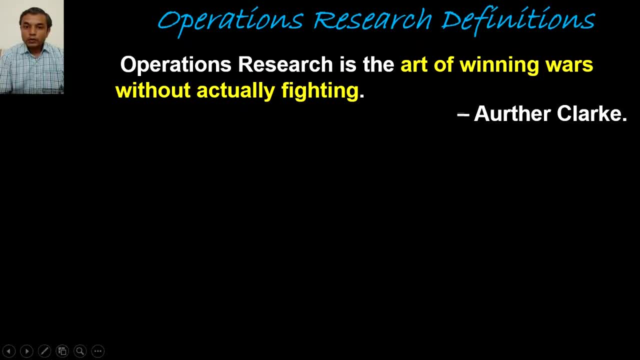 so it's do not actually throw light on operations research technique, but the depth. it is defined on the base of how it is evolved that operations research is a technique where we can maximum utilize our resources, and by utilizing the resources in more, better way, we can get major output. and so, without actually fighting the war, we can have a. 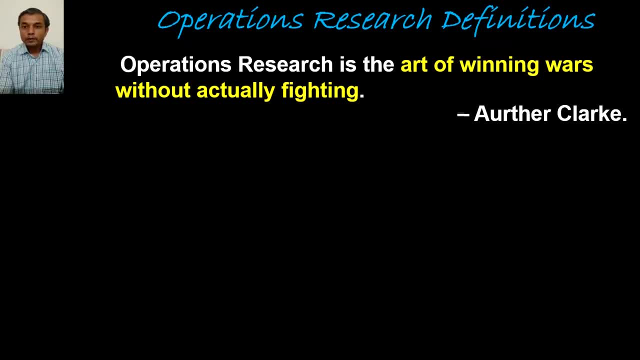 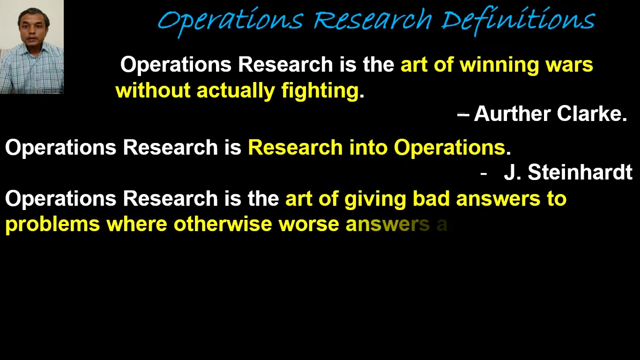 situation where we can win the war. so another definition is operations research is research into operations, here the operations termed in the form of various industrial complex situations, research projects and military operations. operations research is the art of giving bad answers to problems where otherwise worse answers are given. so operations research is the technique used for very complex problems. remember this. 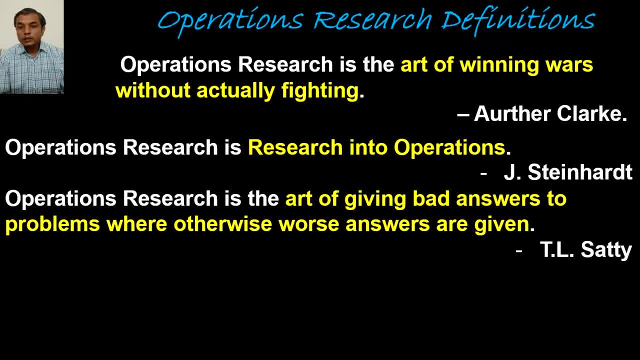 operations research is always used in complex situation. when the same situation is simple and we have answers in easy way. operations research techniques are not advised. it is used in a complex situation when there are so many variables are present and there are so many constraints, and within these constraints we have to get some good answer. so operations- 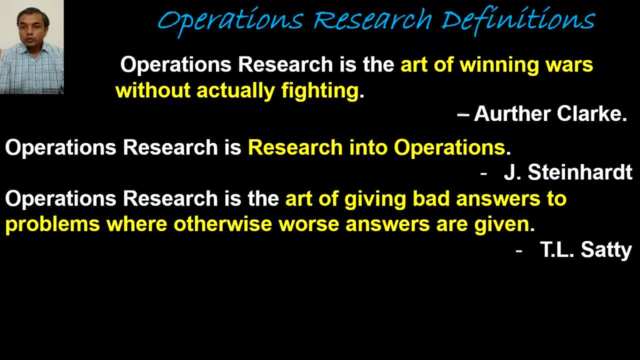 research is used in a complex situation where, if we do not use the operations research, the answer is the worst one and by utilizing the operations research techniques we have some good answers or good output. so it is said that operations research is the art of giving bad answers to the problems where otherwise first answers are given. another definition is: 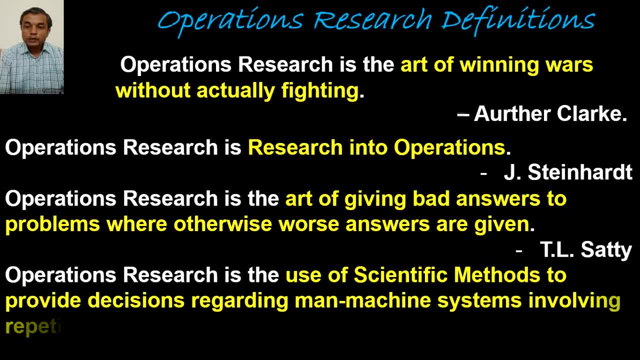 operations research is the use of scientific methods to provide decision regarding main machine systems involving repetitive operations in complex situations. so operations research is applied mathematical techniques and scientific methods to provide decisions regarding main machine systems involving repetitive operations in complete complex situations. so it is regarding the applications of operations research in industries and in industrial complex problems. let's see the. 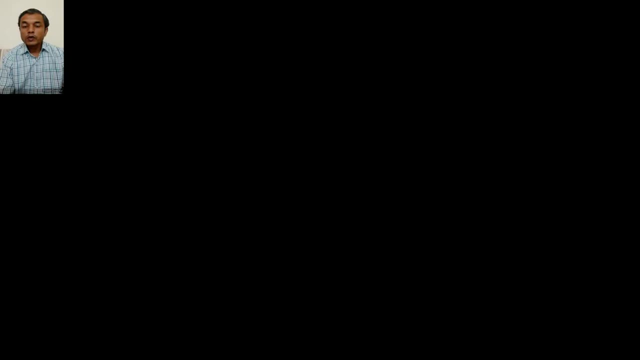 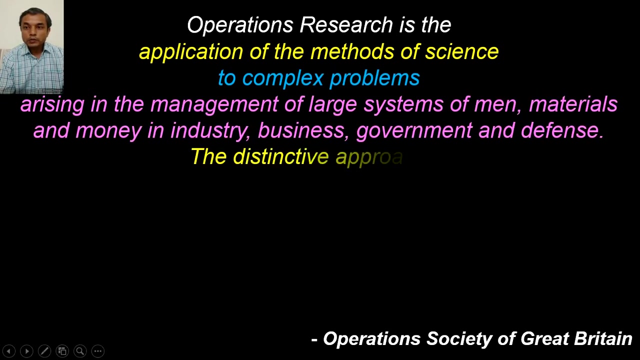 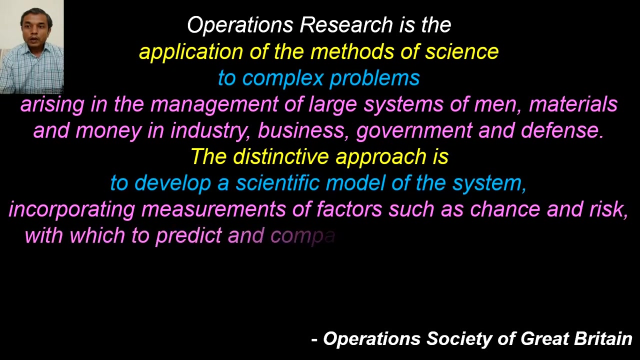 more comprehensive definition of operations research given by operations society of great britain. operations research is the application of methods of science to complex problems arising in the management of large systems of men, materials and money in industry, business, government and defense. the distinctive approach is to develop scientific 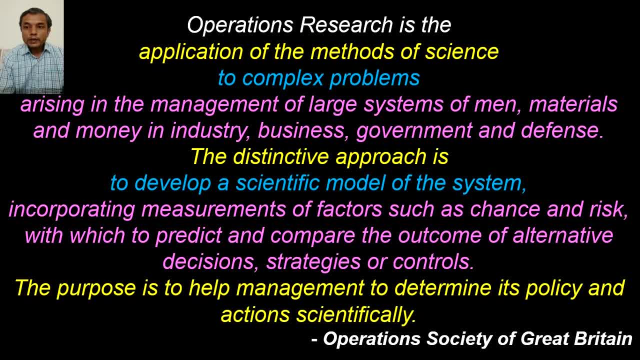 model of the system incorporating measurements of factors such as chance and risk with which to predict and compare the outcome of alternative decisions, strategies and controls. the purpose is to help management to determine its policy and actions scientifically. so this definition is divided into the three part. first part: focus on the 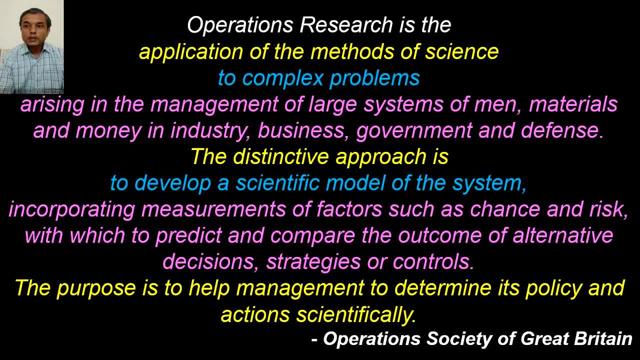 applications of operations research. operations research is applied to only complex problems, as we have discussed earlier, complex problem of management in large systems of men, materials and money, and the area of applications are industry, business, government, defense and research and development. second part of the definition said that it is a scientific. 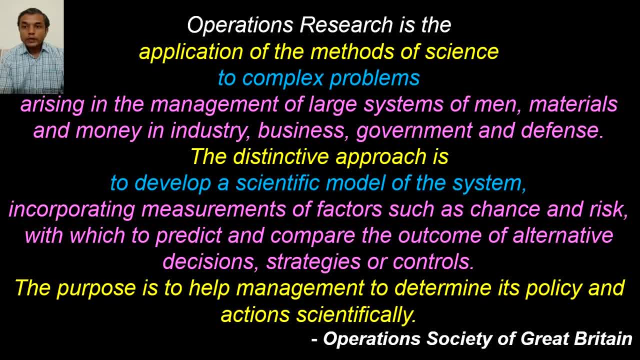 model applied mathematics techniques, which incorporate measurement of factors such as chance and risk, through which predict and compare the outcome of alternative decisions, strategies or control operations. research provide the multiple decisions that are known as a feasible solutions, from which we have to choose a optimum one. and, lastly, 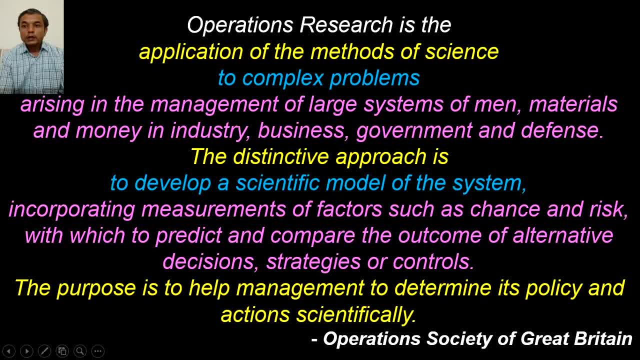 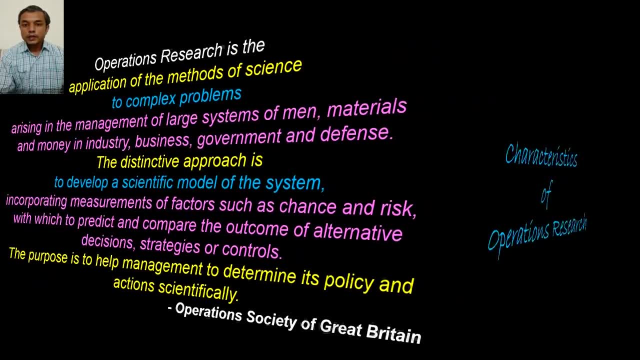 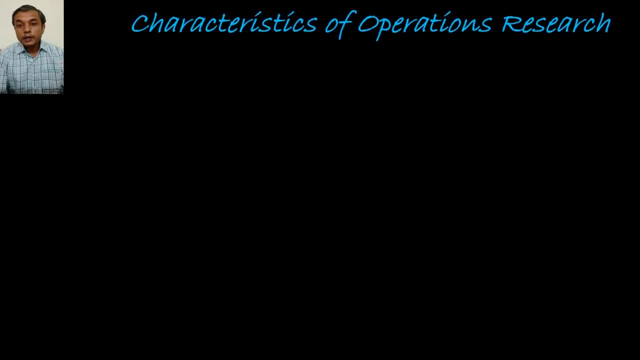 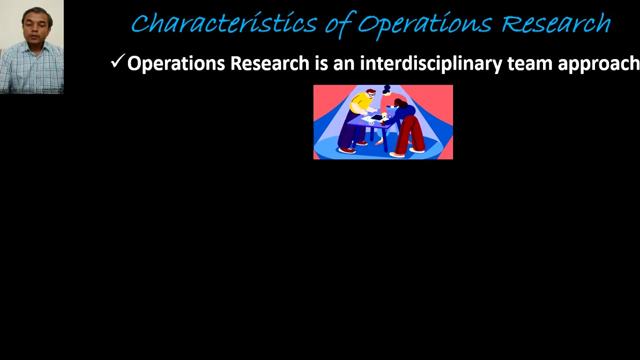 focus on the purpose of the operations. operations research, that to help management to determine its policy and actions scientifically. that is for long term as well as for short term. so this is operations research. now let's discuss characteristics of operations research. operations research is an interdisciplinary team approach. it means saying any industry. there is one problem which is being studied. 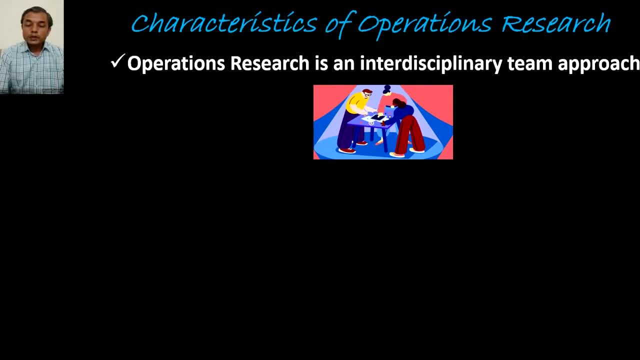 by operations research. so for solving this problem, the members from purchase department, production department, utility department, maintenance section and marketing all are together and then focus on the problem from the all aspects. so So it's an interdisciplinary approach. Operations research increase the creative ability of decision makers. 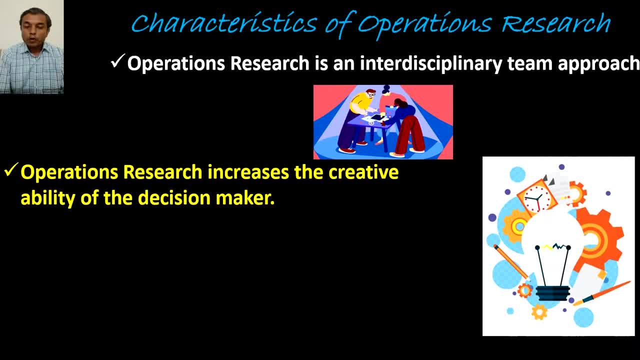 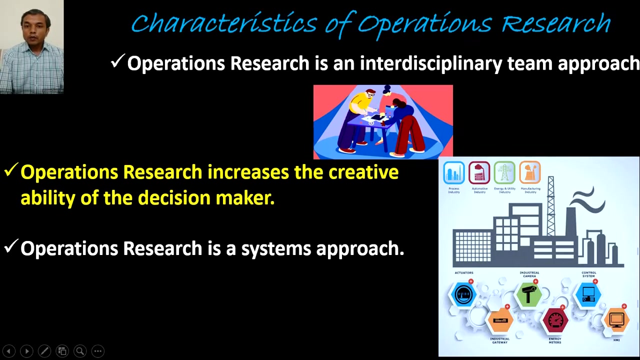 Operations research focus on the multiple solutions, possible, feasible solutions. It thinks on different ways and evaluate the results. So, instead of taking a thumb rule type decision making and conventional decision making, operations research focus on creative ability of thinking for decision makers. Operations research is a system approach as it work in a holistic manner. 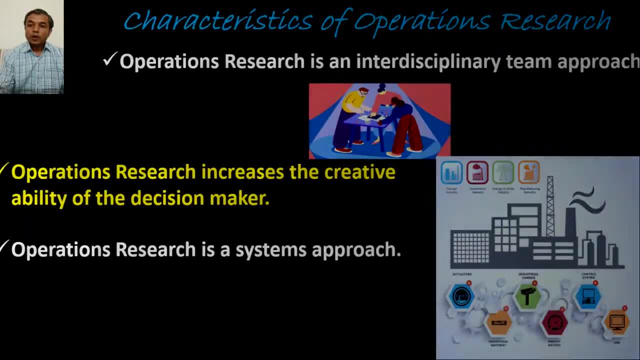 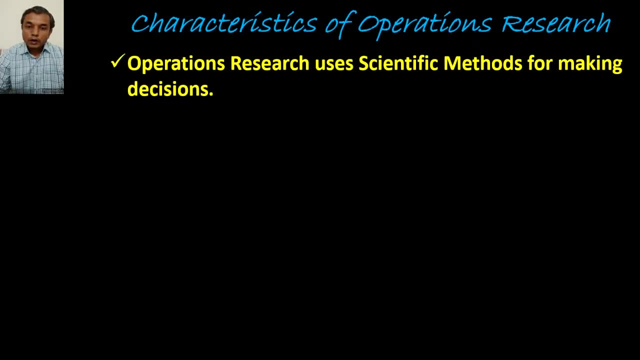 We can say that it is a system approach. Operations research use scientific method for making decisions. Operations research is basically a bunch of optimization techniques. It's the applied mathematics techniques, And so it is a scientific method. So it's a bunch of optimization techniques. 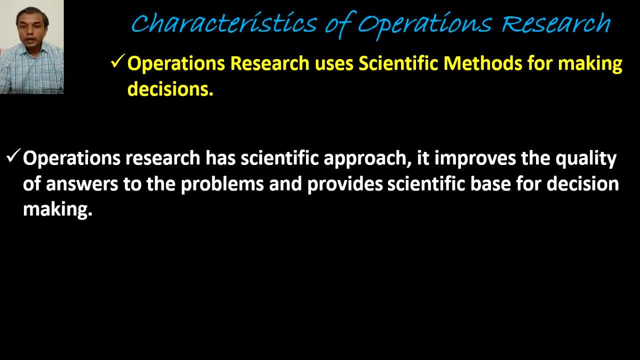 So it's a scientific way of decision making. It's not gazing and predicting. Operations research has scientific approach. It improves the quality of answers to the problem and provide scientific ways for decision making. Operations research provides the effect of various variables on the result. 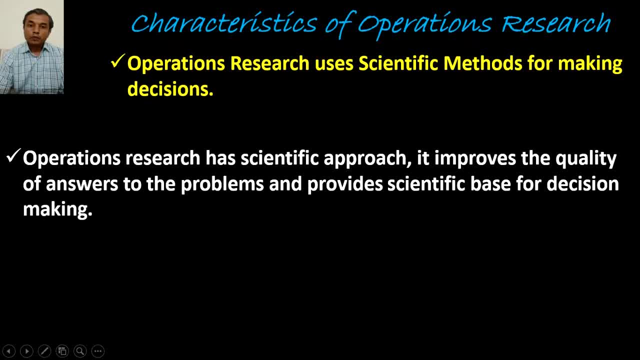 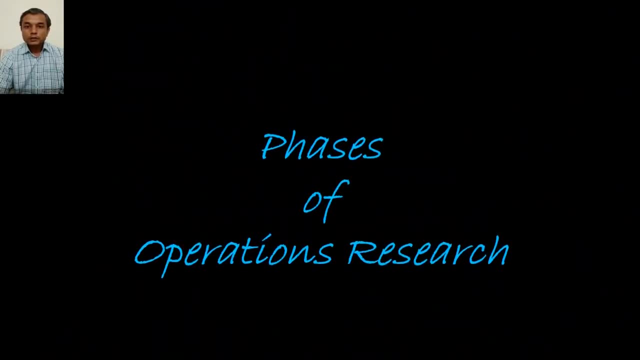 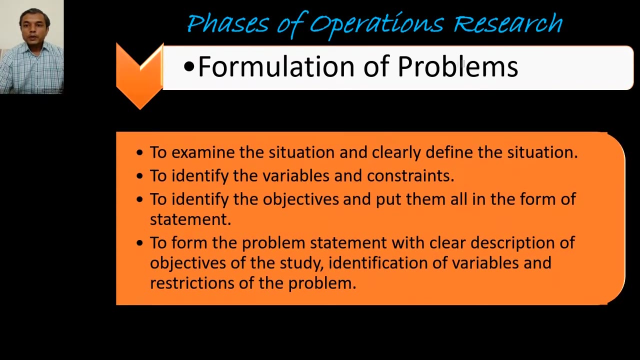 We can have a sensitivity analysis, that what is the effect of various variables on the output. So on the basis of that, managers can take better decisions. Now let's discuss phases of operations research. First phase of operations research is formulation of problems. So first is to examine the situation and clearly define the situation. 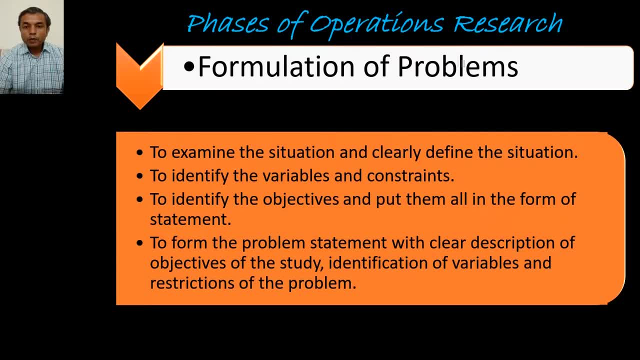 First, focus on the problem and study the problem. to identify the variable and constraints within the problem problems. to identify the objectives and put them all in one statement that is known as a formulation of the problem in verbal form. to form the problem statement with clear description. 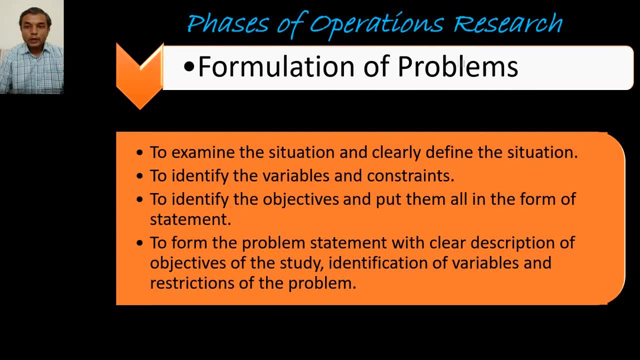 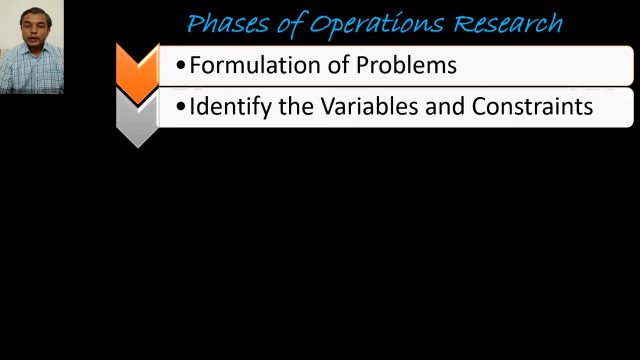 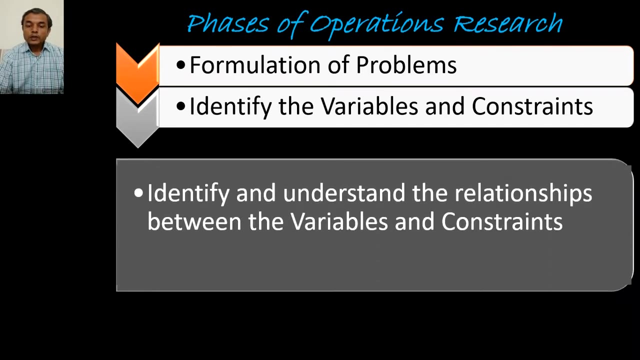 of objectives of the study, identification of variables and restriction of the problem. so in this first step of formulation of the problem we convert the situations in the verbal form in very clear and precise way. next step is the identify the variables and constraints. so in this phase we identify the variables, constraints and establish the relationships. 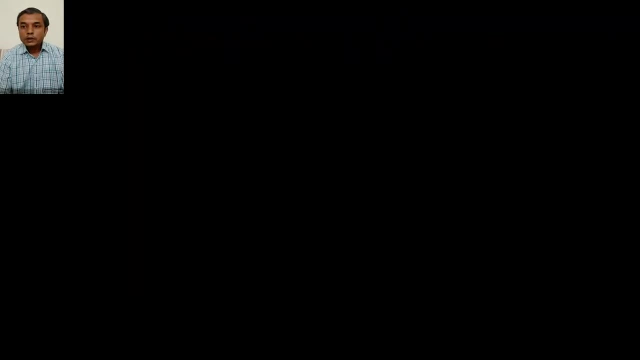 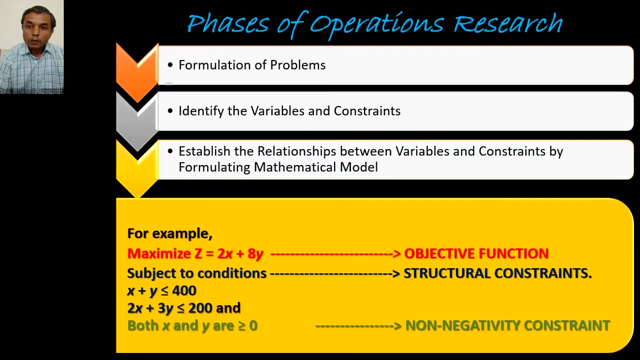 between the variables and constraints. next step is establish relationship between variables and constraints by formulating mathematical problem. for example: maximize z equal to 2x plus 8y. so here x and y are the variable and the problem statement is maximization of z 2x plus 8y, subject to: 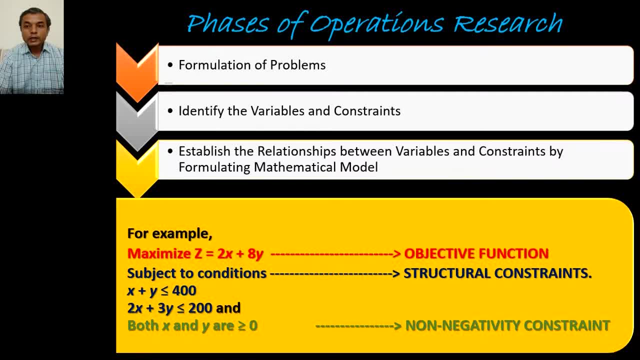 the conditions- these are our structural constraints- that x plus y is less than or equal to 400 and 2x plus 3y is less than and equal to 200. both x and y are greater than or equal to zero. these are the non-negative constraints. so it is a formulation of problem into mathematical form. 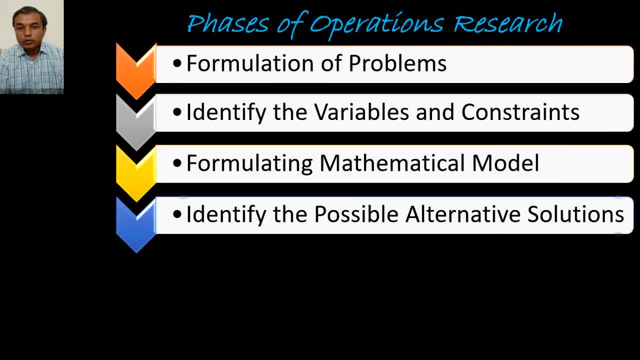 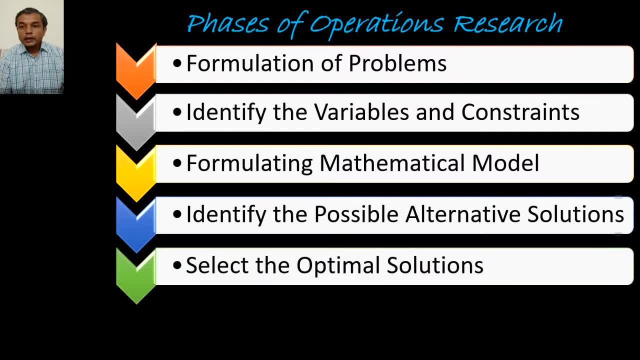 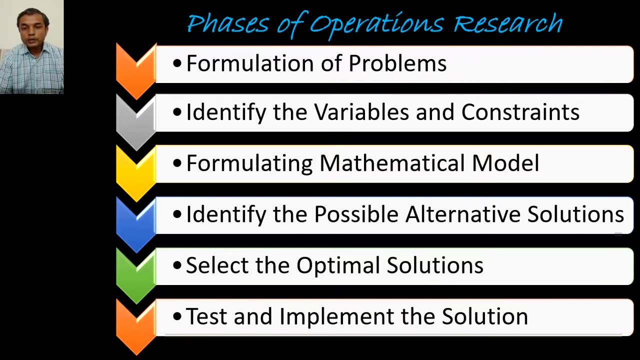 after that, next step is identify the possible alternative solutions by solving this problem, so these are known as a feasible solutions. then next step is select the optimal solutions among the possible visible solutions. then test and implement the solution. so these are the phases of operations: research, that how operational research. 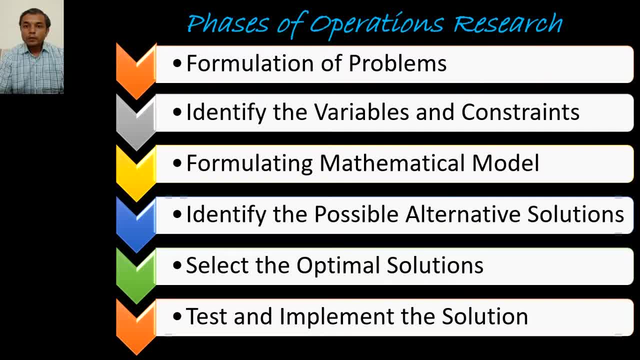 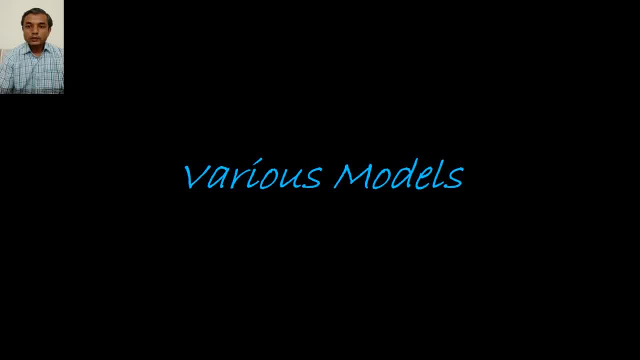 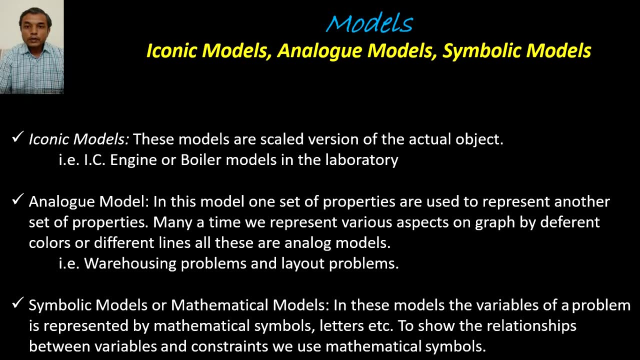 techniques work, and this is applicable to all techniques of operations research. now let's discuss various models of operations research. the first is iconic models and symbolic models. iconic models are the models which are the scaled version of the actual object, so in other sense we can say that these are the prototype. for example, in our laboratories we have 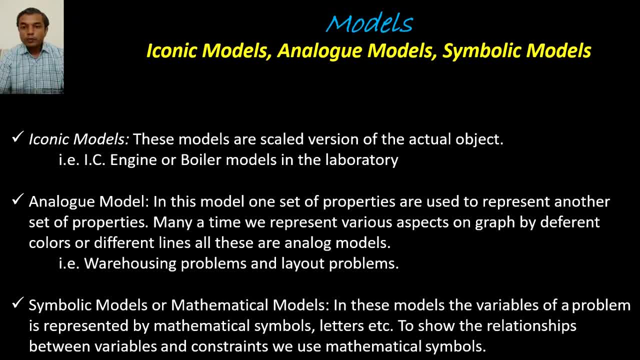 ic engine or boiler models. so these are the prototype of actual ic engine or boilers. so these are known as iconic models. analog model: in this model, one set of properties are used to represent another set of properties. many times we represent various aspects on graph by different colors. 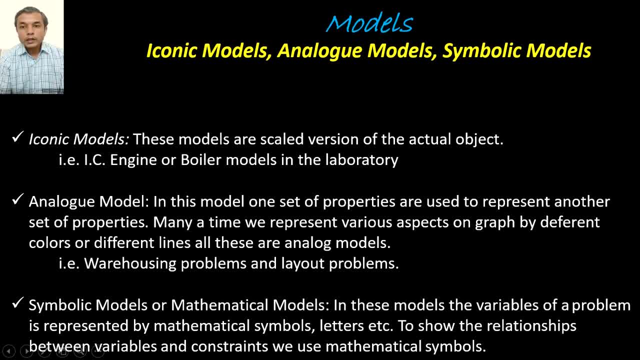 or different lines. all these are analog models. for example, normally we represent water by blue color, so on map water is represented by blue color. river sea are represented by blue color. so this is the example of analog model. another example is warehousing problem and layout problems, where we use analog model. other model is symbolic or 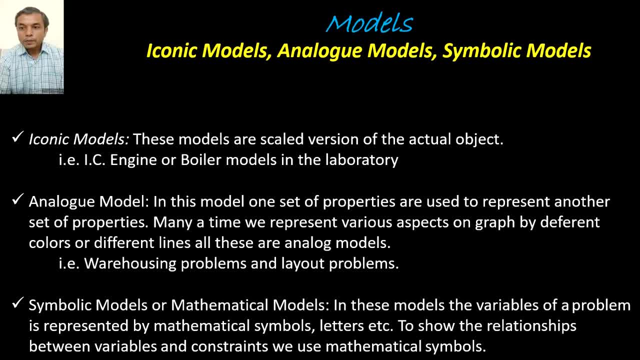 mathematical model. this is used in operations research. in these models the variables of problem is represented by mathematical symbols- letters etc. to show the relationship between the mathematical and the mathematical constraints we use as a mathematical symbols. so in previous form, previous discussion- we have discussed that in phases of operations research we form the 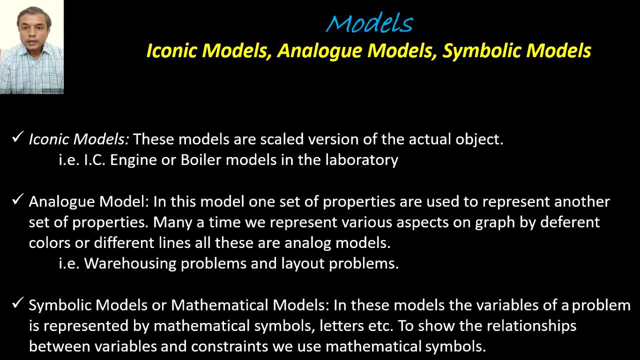 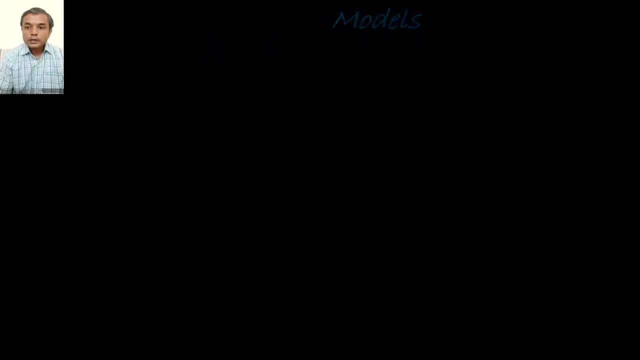 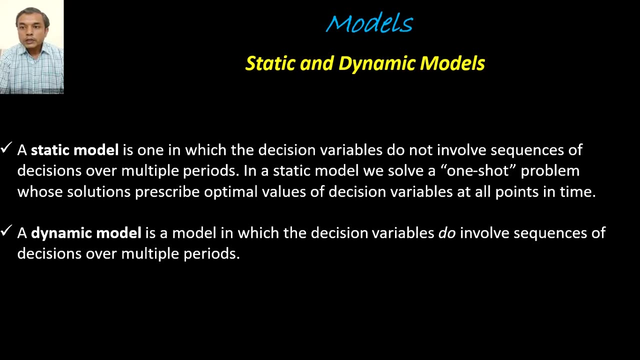 numerical form of problems. say: maximize z is equal to 2x plus 8y, subject to 3x plus 4y greater than or equal to 20.. so it is an example of mathematical model. next is static and dynamic model. a static model is one in which the decision variables do. 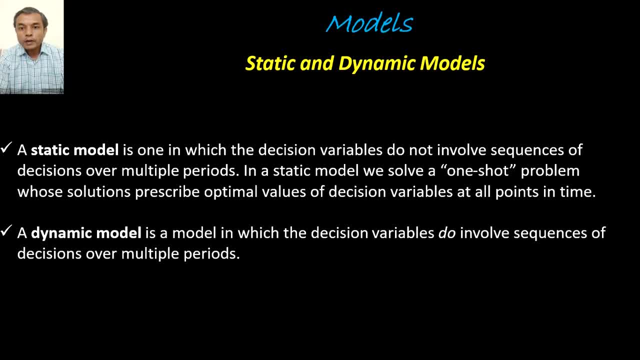 not involve sequence of decisions over multiple periods. in static model we solve a one short problem whose solutions prescribe optimal values of decision variables at all points in time. so static model does not vary with both VAN. so static model is a style for its flow, the dynamic model is a model. 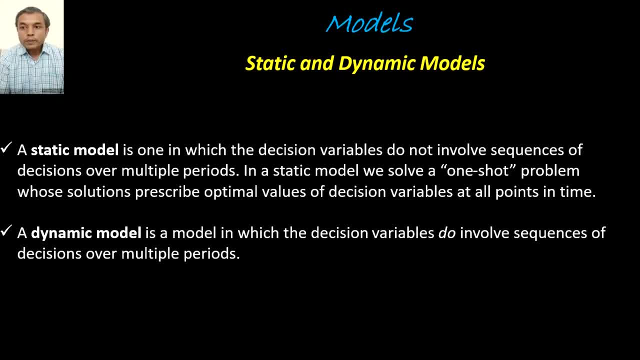 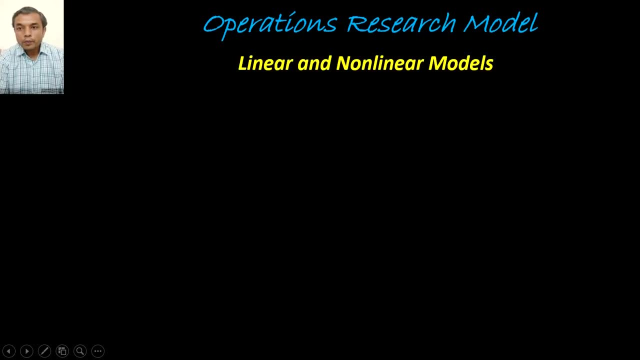 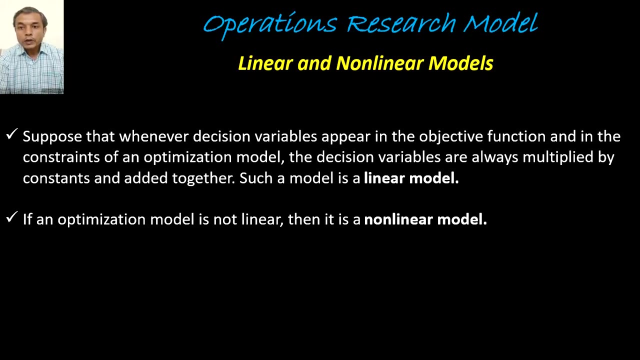 in which the decision variables do involve sequence of decisions over multiple periods. it change with time. so that is staticoused dynamic models. another is linear and non- nunca, with states of developers and production teams. linear models Suppose that whenever decision variables appear in the objective function, 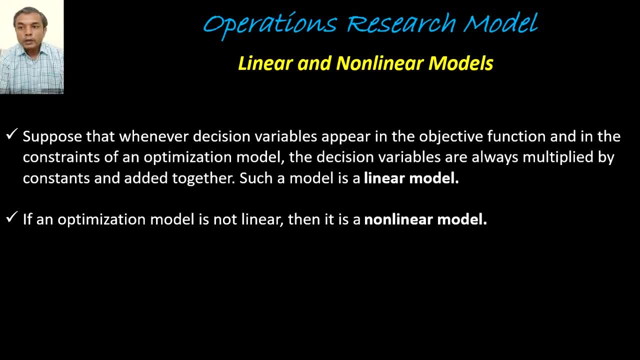 and in the constraints of an optimization model, the decision variables are always multiplied by constants and added together. Such a model is a linear model. In other sense, the relationship between variables is linear: The decrease in one variable, the effect on another variable. 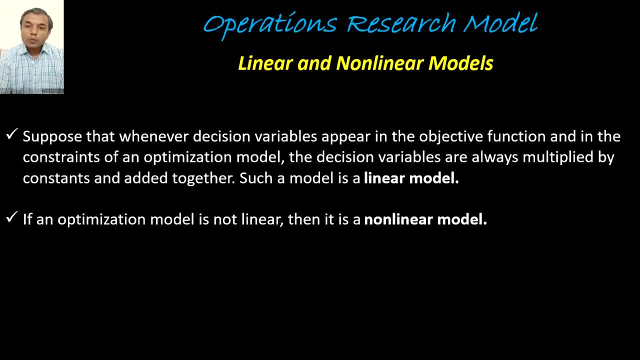 is in a linearity form. Such kind of model is known as a linear form. When the relationship is not linear between variables, such optimization model is known as a non-linear model. In operations research we will discuss both linear models and non-linear models. 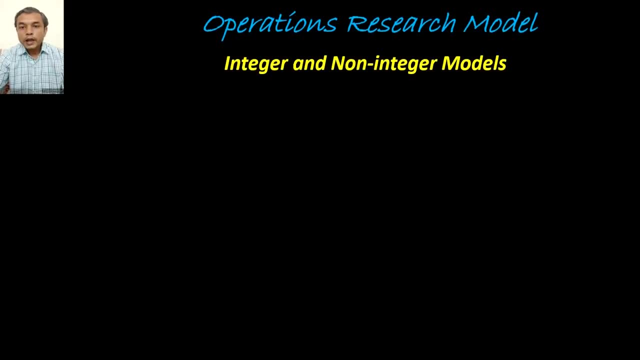 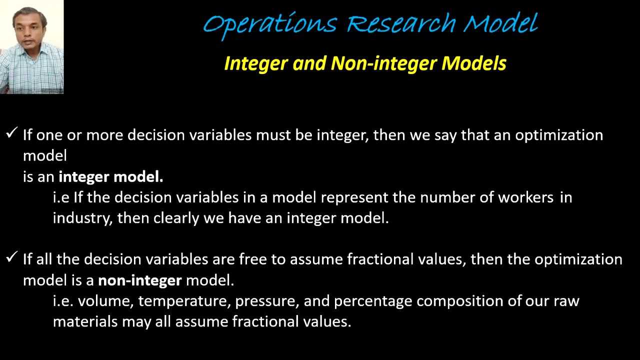 Next is integer and non-integer models. If one or more decision variables must be integer, then we say that optimization model is an integer model. For example, if the decision variable in the model represents the number of workers in industry, then clearly we have 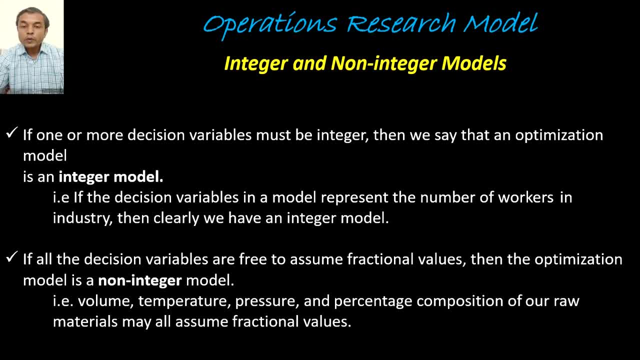 an integer model, Because we cannot have 1.5 workers. we can't have 1.5 workers or 20.2 workers. It is either 20 or 21. So such kind of model is known as integer model. 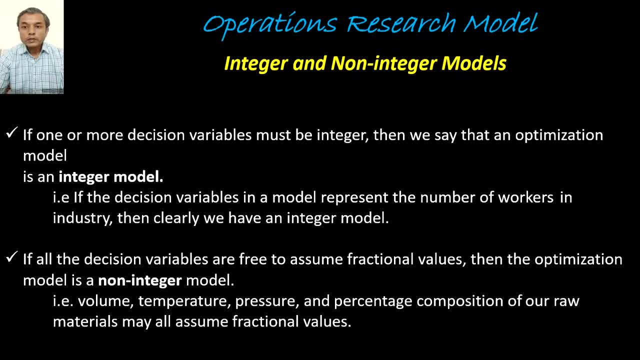 Non-integer model, in which the decision variables are free to assume fractional values. Then the optimization model is known as non-integer model. For example, volume, temperature, pressure and percentage composition of raw materials. All these are an example of non-integer variables. 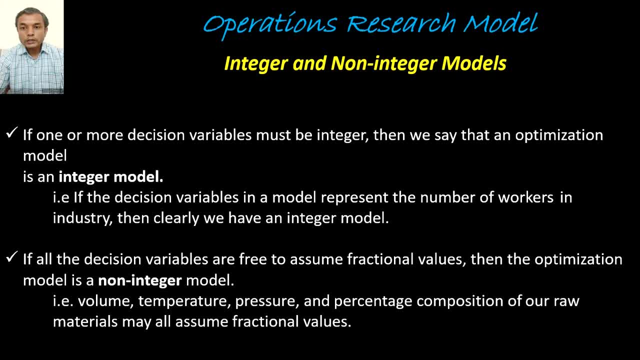 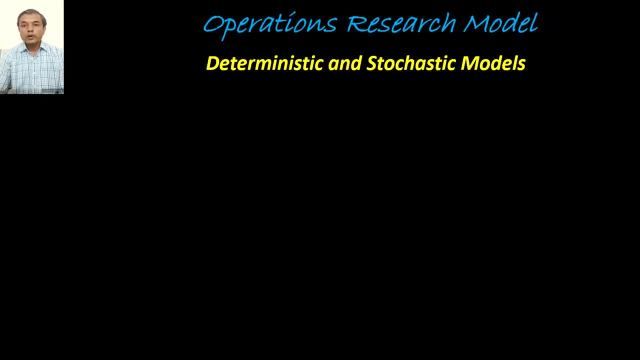 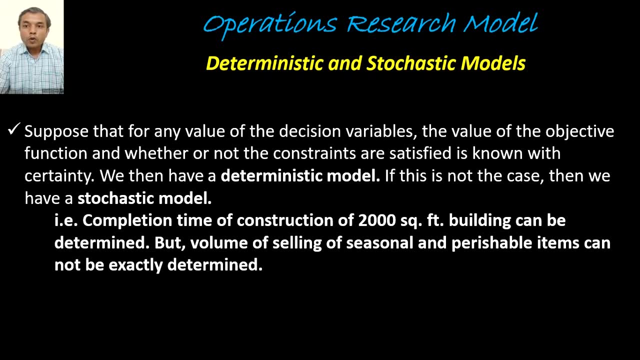 In operations research. we will discuss both integer and non-integer models. Next is deterministic and stochastic models. Suppose that for any value of the decision variables, the value of objective function and whether or not the constraints are satisfied is known with certainty. We then have a deterministic model. 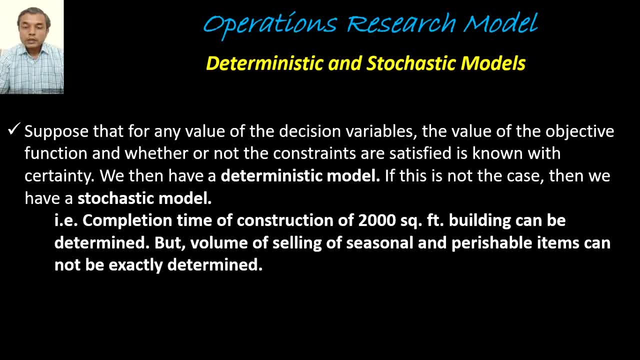 If this is not the case, then the model is stochastic model. For example, completion time for the construction of 2000 square foot building can be determined Because we know that 10 workers can build this much amount of building or this much amount of volume in one day. 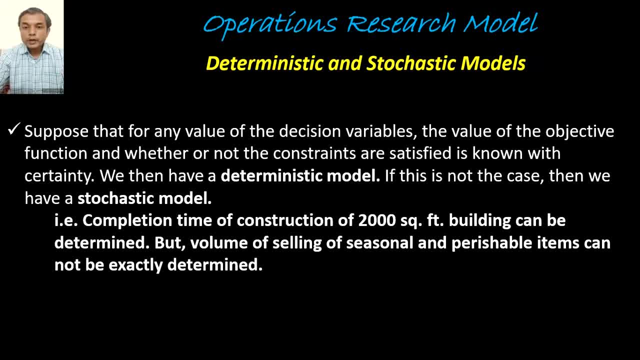 So with the help of such database, such determined database, we can calculate the total duration of the project. So such kind of model is known as a deterministic model. In another sense, if a worker can make 10 jobs in one shift, then we can say that in 5 shifts worker can make 50 jobs. 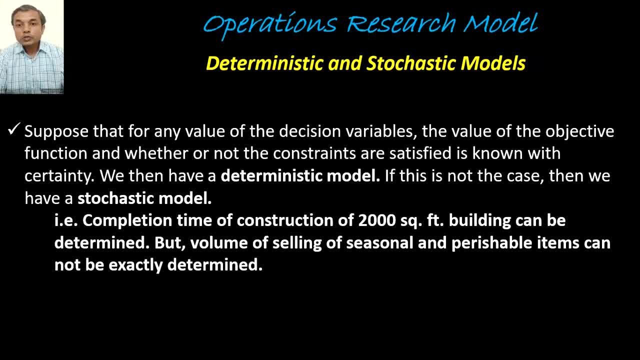 So it is a deterministic model. But the situation where we cannot determine the exact amount of value, Like in case of seasonal products and perishable products, the amount of sale of the product we cannot exactly determine. So such kind of problems are dealt in stochastic model. 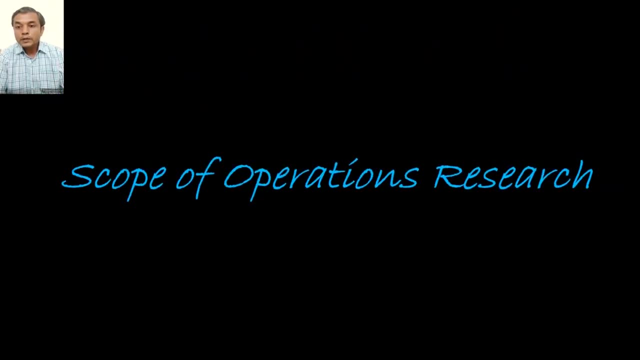 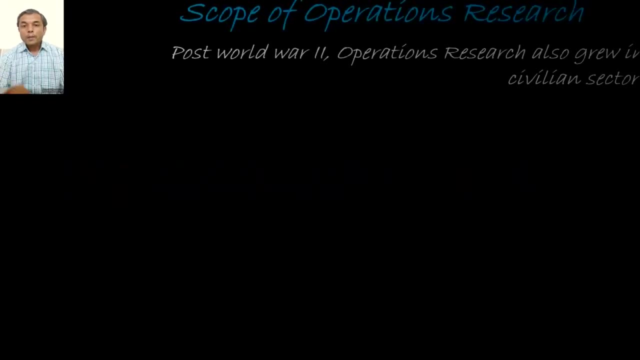 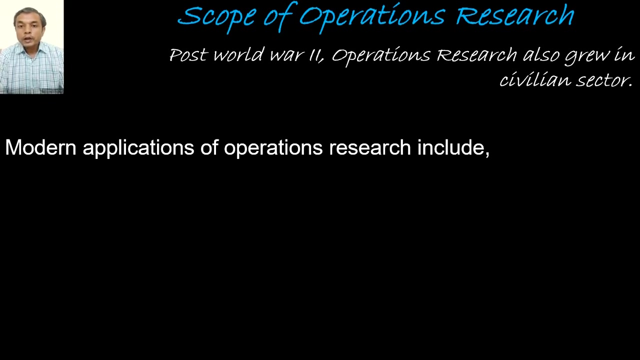 So these are the various models used in operations research. Now let's discuss scope of operations research After World War II. so we can say that in post-World War II operations research is also growing. In civilian sector operations research is adopted by industries, research and development organizations, government and so on. 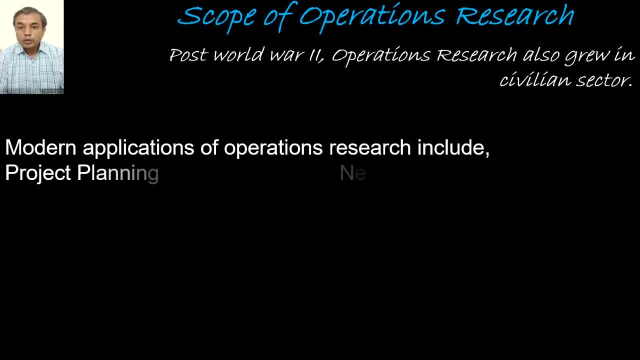 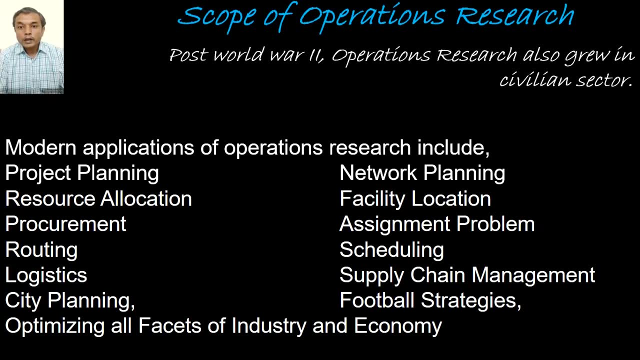 So nowadays operations research is used in project planning, network planning, resource allocations, facility locations, procurement in assignment, problem routing, problem scheduling, logistics, supply chain management, city planning, football strategies, Optimizing all facets of industry and economy. 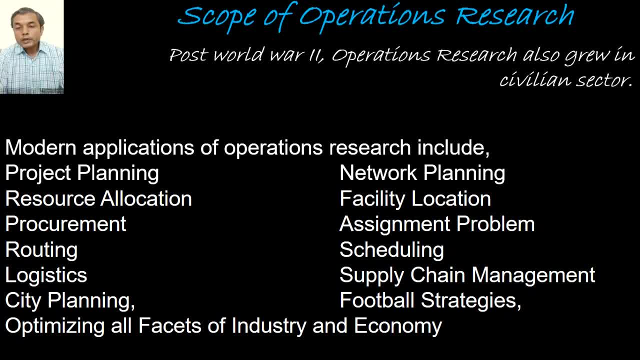 So operations research is used in almost all area of industries: for strategic decisions, for software decisions and medium term decisions. So as computing technologies develop day by day, the use of operations research is also increased, Because we can easily develop the relationship among various variables and constraints and then we can come to some decisions.